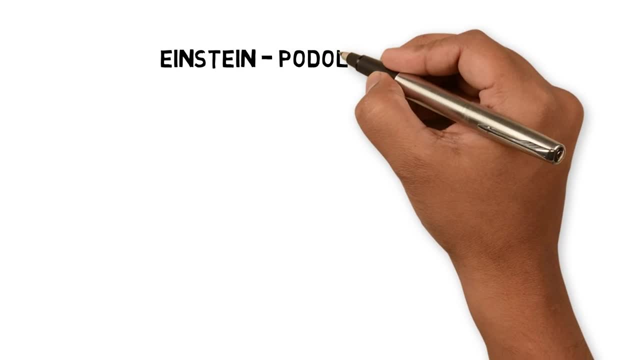 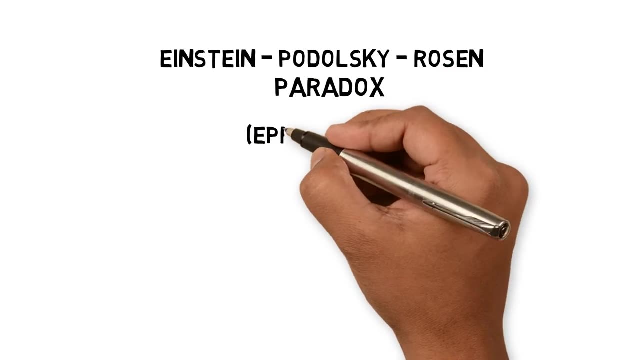 Complementarity does not always involve a one-or-the-other relation. however, In 1935, in an influential thought experiment, known as the Einstein-Poldol-C-Rosen paradox arose. Einstein believed that some particles could move in such a way that it was possible to measure their position and momentum. 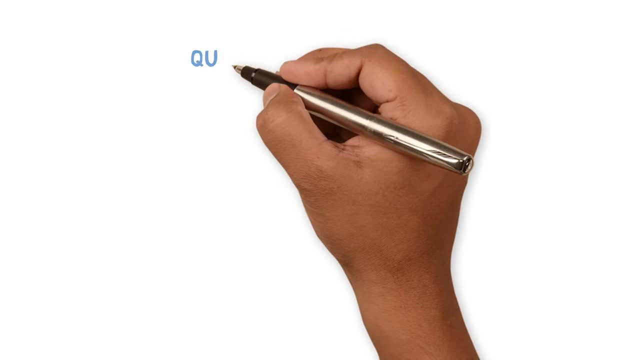 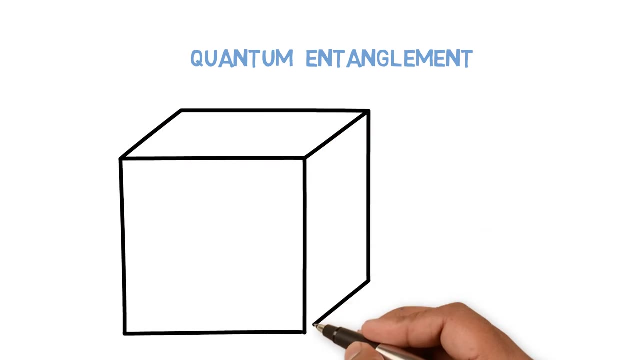 more accurately. This is where quantum entanglement comes in. The meaning of this is essentially in the term itself. Entanglement describes a phenomenon where two objects act on each other and become an entangled system. Imagine there is one child in the room and you know that the total 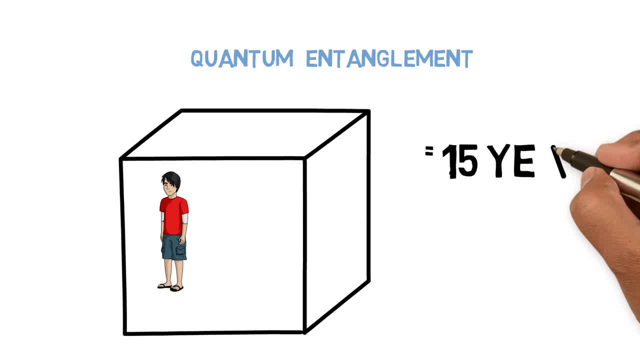 age in the room is 15.. Clearly the child is 15 years old. Now what if I told you that there were two children in the room and the total age was 15? Find the age of each child. The answer is impossible to find. There are many, many possibilities. Now place this concept into that. 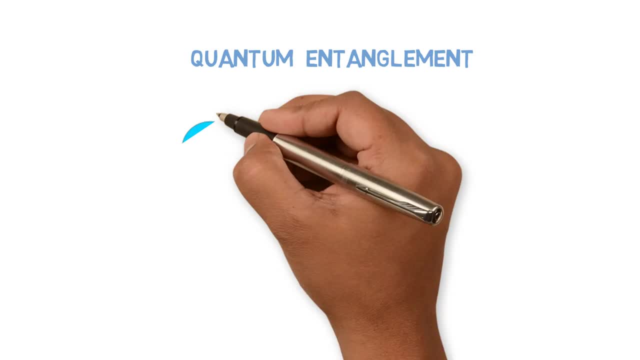 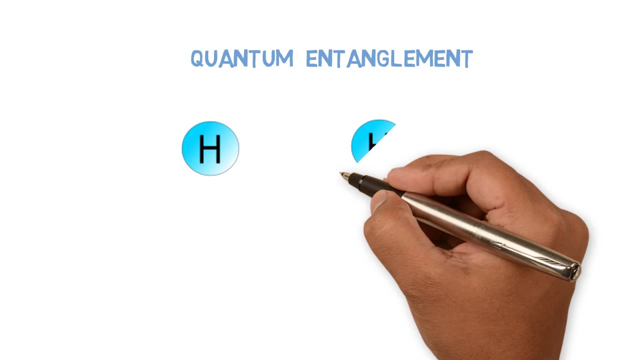 of particles. Let's say we have a single hydrogen atom. From observing said atom we can determine its position, spin, momentum, energy and other variables. Now imagine you have the same data, except it's for two combined hydrogen atoms. It would be impossible to determine the properties. 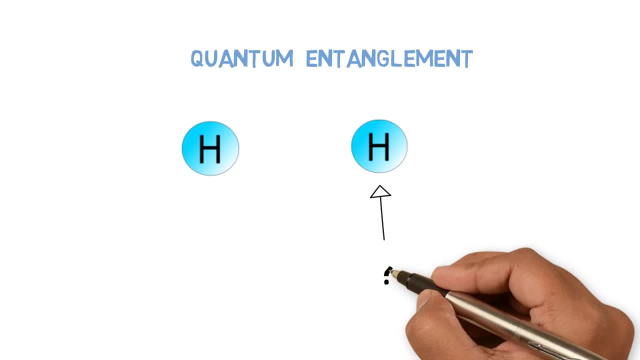 of each individual atom in the pair. Hence, the data can only be described as a whole, no matter how far these particles are from each other. Another example of complementarity is that of waves and particles Known as wave-particle duality. this principle states that when 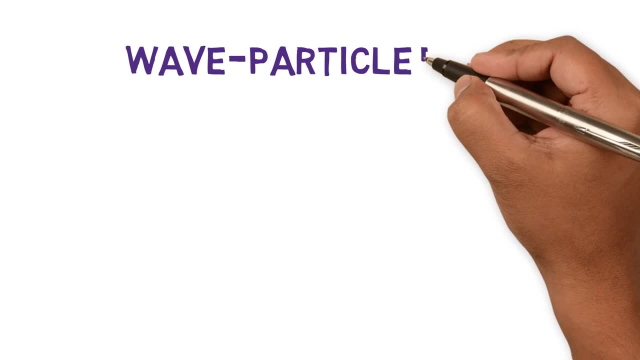 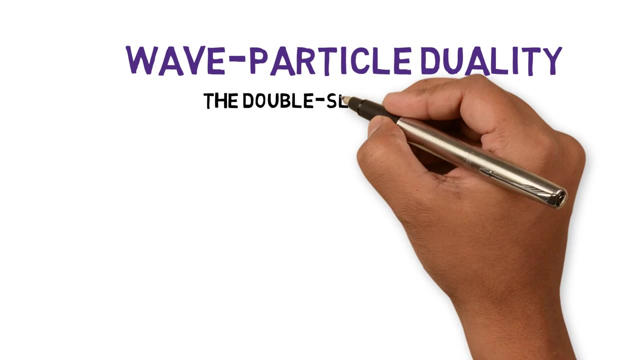 describing any elementary particle, a wave-particle duality is a wave-particle duality or any entity, you must describe it as both a wave and a particle. However, both states cannot be observed at once. This concept can be explained by the famous double slit experiment originally. 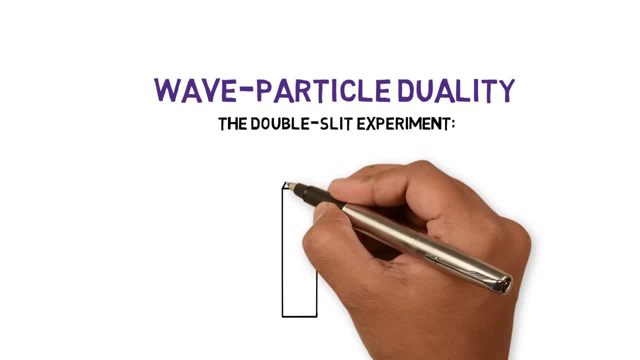 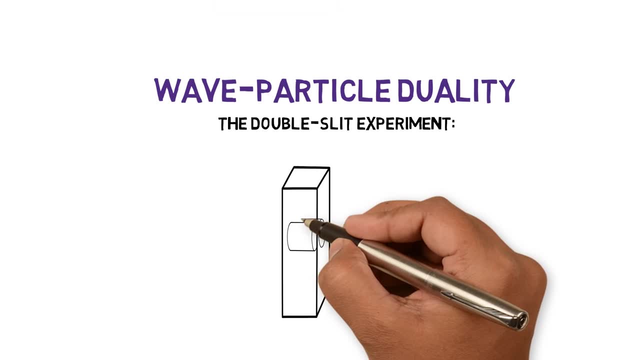 designed by Thomas Young. First light, preferably laser light, is directed through two holes that are next to each other. When the light passes through it, it creates an interference pattern, direct evidence that it is a wave. However, when observed through a light-sensitive camera, 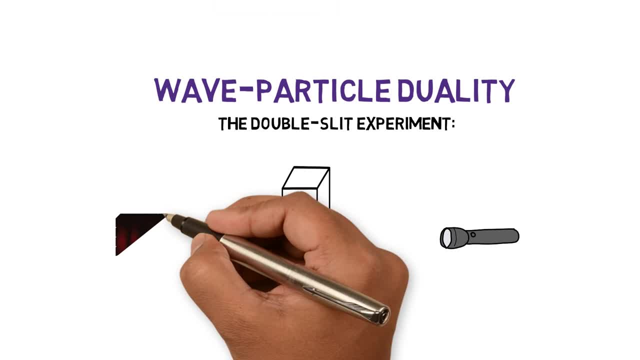 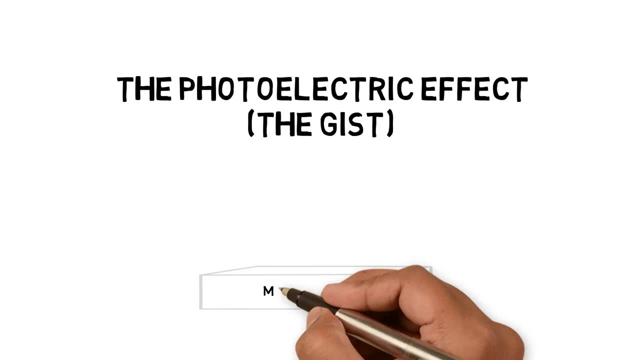 one would see pinpoints, thus proving it's made of particles. Although scientists are uncertain of how this is possible, numerous experiments have proven this theory. In yet another famous experiment known as the photoelectric effect, Einstein showed that when photons at a high enough energy were hit against metal, they were able to push off electrons from. 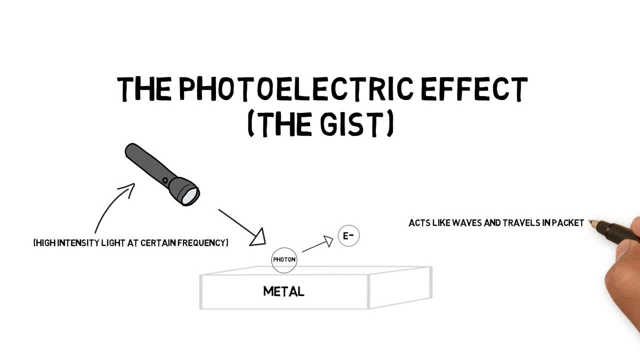 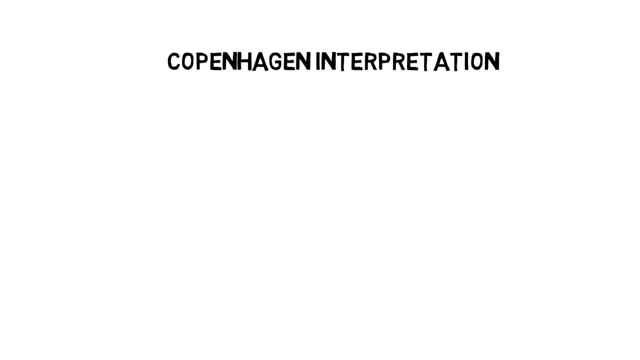 the surface. He showed that photons can move in waves but at the same time travel in packets known as quanta. These principles fall under the Copenhagen interpretation of quantum physics. In summary, physical systems do not have definitive properties and quantum mechanics can only provide probabilities. However, when these properties are actually measured, the number